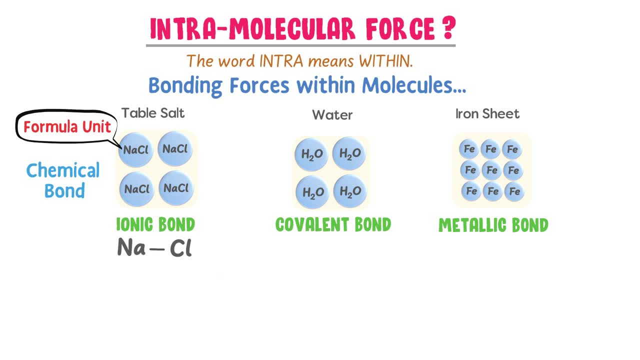 chemically bonded to chlorine atom due to ionic bond. Sodium atom is chemically bonded to chlorine atom due to ionic bond. Sodium atom is chemically bonded to chlorine atom due to ionic bond. Sodium atom is chemically bonded to chlorine atom due to ionic bond. So the bonding force within 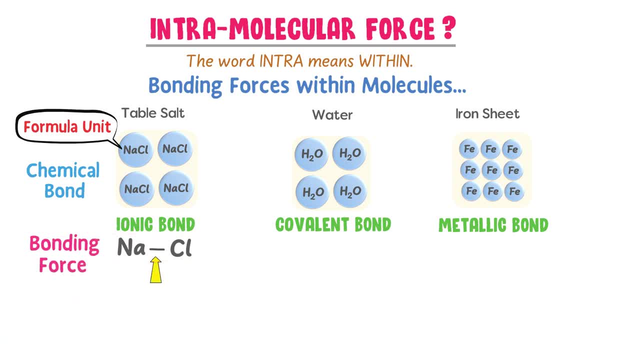 formula unit of sodium chloride is called as intramolecular forces. Thus here intramolecular forces exist within formula unit. Secondly, the smallest unit of covalent compounds is a molecule like H2O. We know that oxygen atom shares two electrons with each hydrogen atom, So 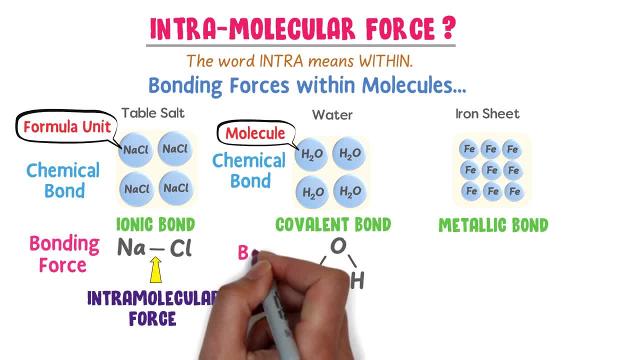 we know that sodium atom cause alpha capose covalent FeClto to make. it is joined from the calcium atom and will create an atom worthy. Here we can take the elect techno假 equation and compute the solution in this feeling. So we know that the specialty of NaCl is that itsZY has largerHHC value in its atom than the. 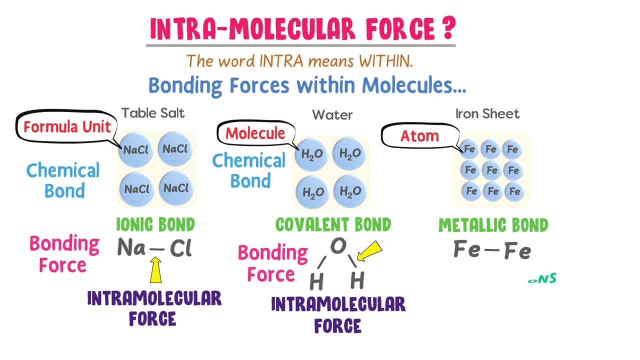 electron所, ions within the lattice. So the bonding force within the iron atom is called as a intramolecular force. Here intramolecular force exists within the lattice. Now listen carefully. We learn that intramolecular forces exist within the formula units of all ionic compounds. Secondly, 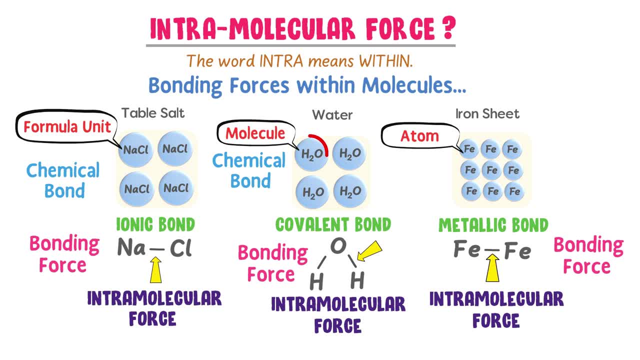 intramolecular forces exist within the molecules of all covalent compounds. Thirdly, intramolecular forces exist within the lattice or sheet of all metallic compounds. Therefore we say that intramolecular forces are the bonding forces within formula, unit, molecule and metals. 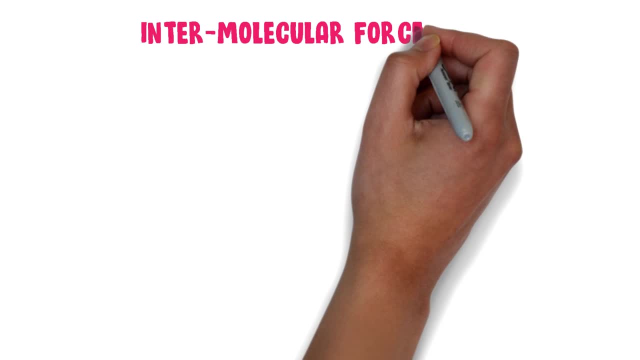 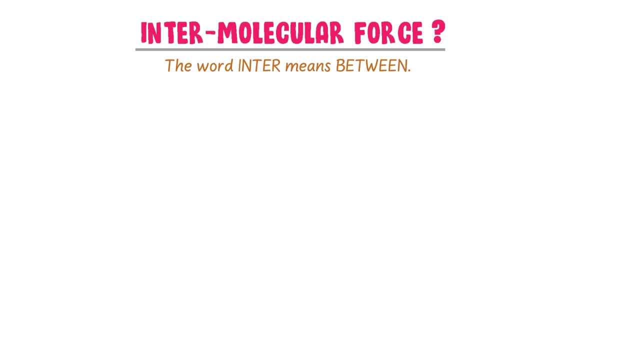 like iron. Now, what are intermolecular forces? Well, the word inter means between. Intermolecular forces are attractive forces between molecules. Usually, intermolecular forces exist and covalent compounds. For example, consider two molecules of hydrogen fluoride and two molecules of water. We know that both in this molecule and in this molecule, 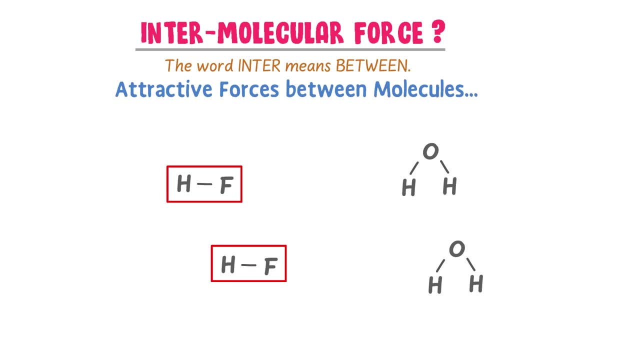 hydrogen is chemically bonded to fluorine atom. We learn that when there is chemical bond, there is bonding force known as an intramolecular force. Thus, intramolecular forces exist within this hydrogen fluoride molecule and also within this hydrogen fluoride molecule. Now let me ask. 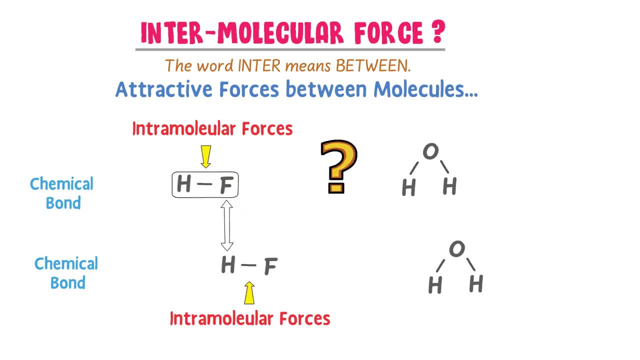 you how this molecule is joined, 1. Why it is created in man. 2. How it is attracted to man. No, it isapi, but we have to understand children born in coming age. So children born in that means. 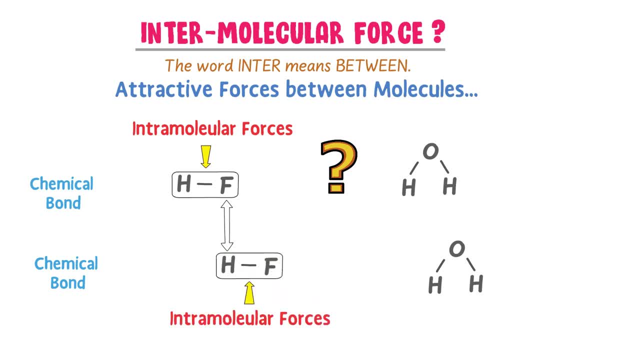 they are attracted to man. So a man. we say that the other person born is a man who lives in other place, which is same age. There is another girl in the world which is the same age. who is the other human? this molecule. Can you guess the answer? Well, this molecule of hydrogen fluoride is attached. 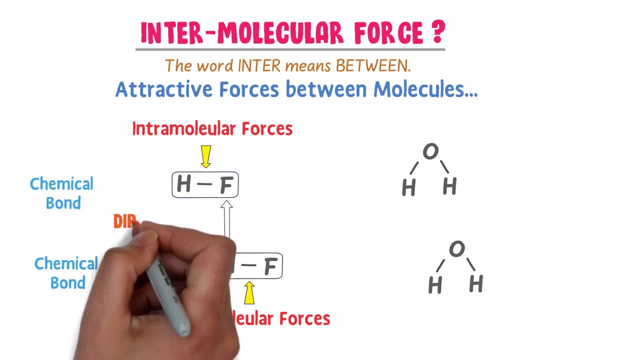 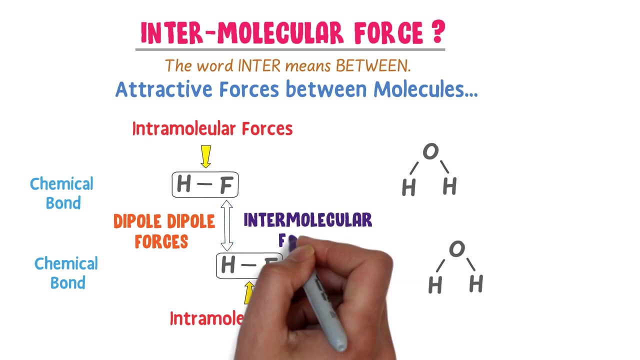 to this hydrogen fluoride molecule due to dipole-dipole forces. Let me repeat it: This molecule of hydrogen fluoride is attached to this hydrogen fluoride molecule due to dipole-dipole forces. We call this dipole-dipole forces between these molecules as intermolecular forces. Hence, 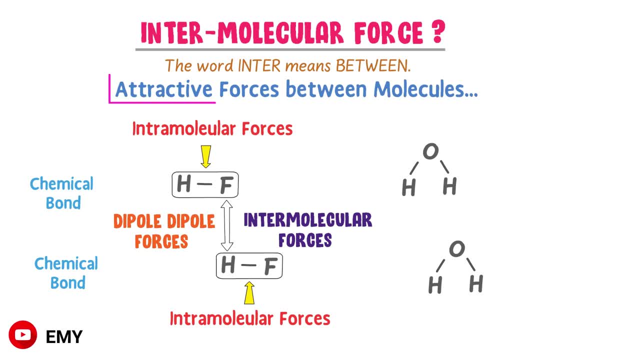 we say that intermolecular forces are the attractive forces between molecules. They are not bonding forces. Secondly, in a single molecule of water there is bonding forces or intramolecular forces within the water, But this water molecule is linked to or attracted by this molecule due to dipole-dipole forces. 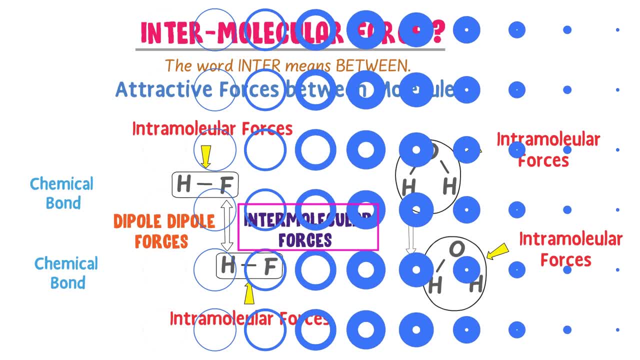 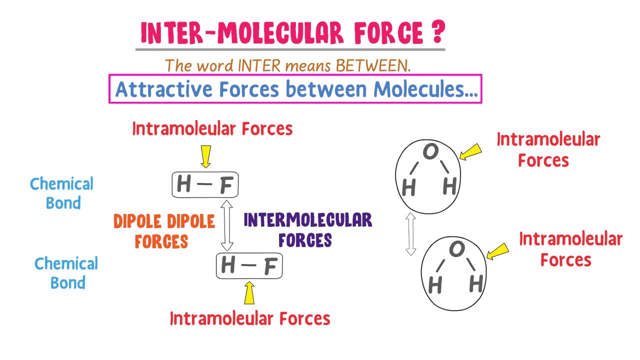 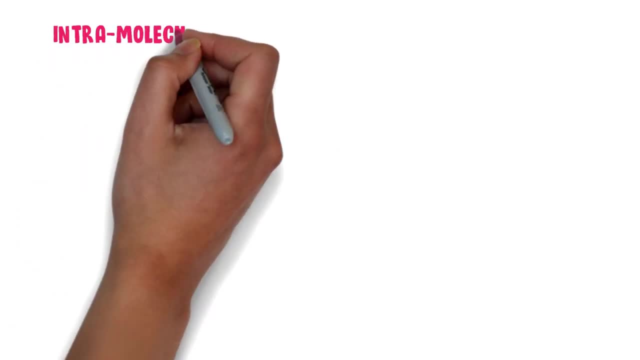 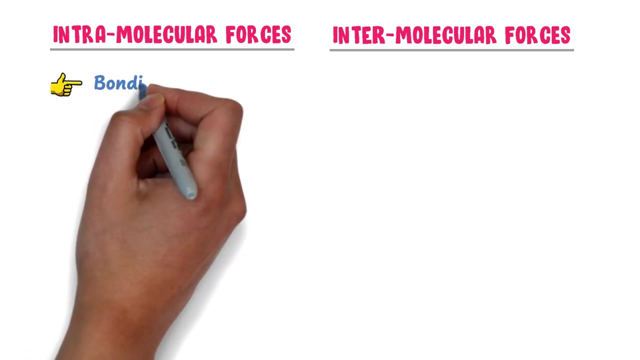 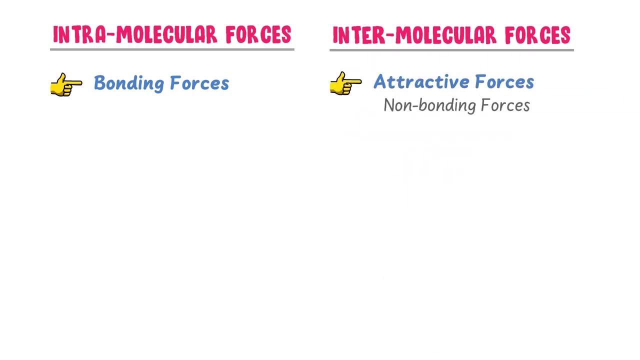 also known as intermolecular forces. Therefore, remember that intermolecular forces are the attractive forces between two or more molecules. Finally, let me teach you the difference between intramolecular forces and intermolecular forces For sequences of interess, under the right person and lower, creating a nuisanceeled 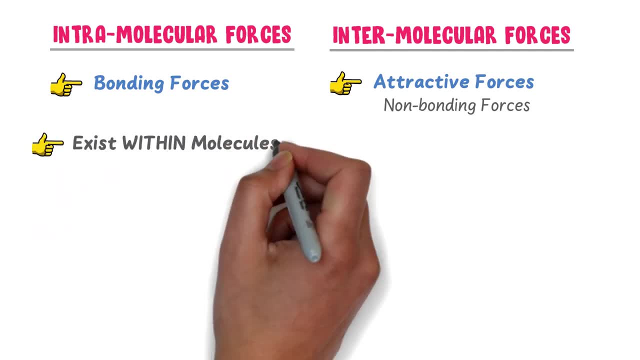 Mask here For capacities of molecules. Intramolecular forces are bonding forces. forgiveness of birlikte out- Pareto kind, full follow through if you are beans. Intramolecular forces are attractive forces or non-bonding forces. Intramolecular forces exist within molecule or formula unit.